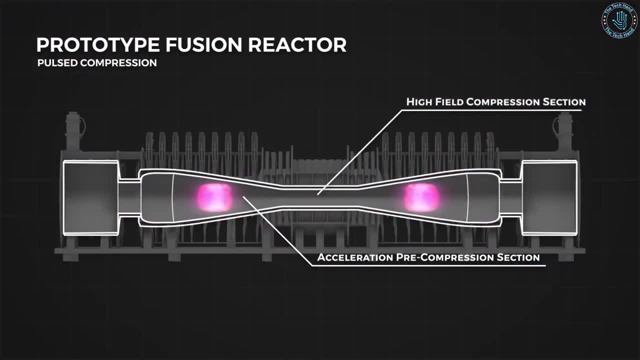 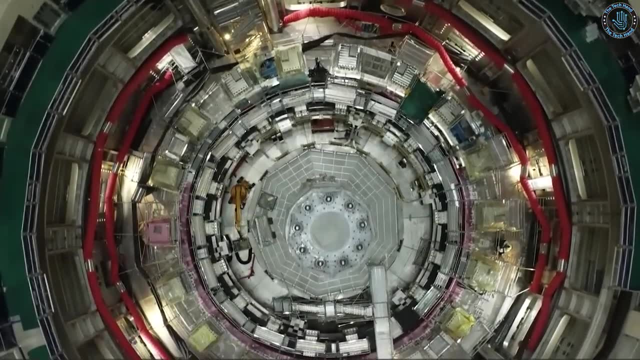 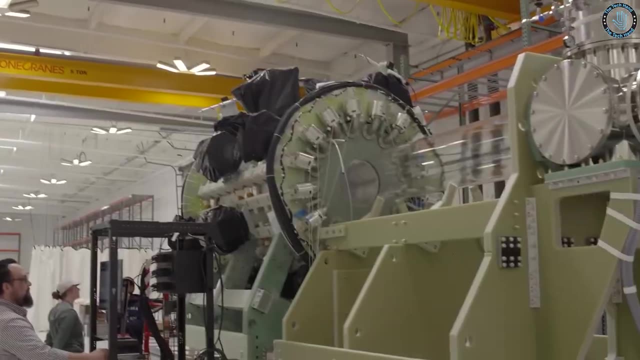 20th century, when scientists first discovered that the nuclei of atoms could be fused together to form heavier elements. In the 1920s and 1930s, physicists began to experiment with ways to achieve nuclear fusion in a controlled environment. The first major breakthrough in the field of nuclear fusion came in the late 1930s. 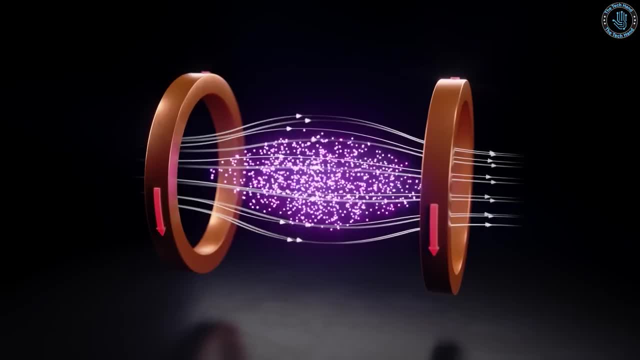 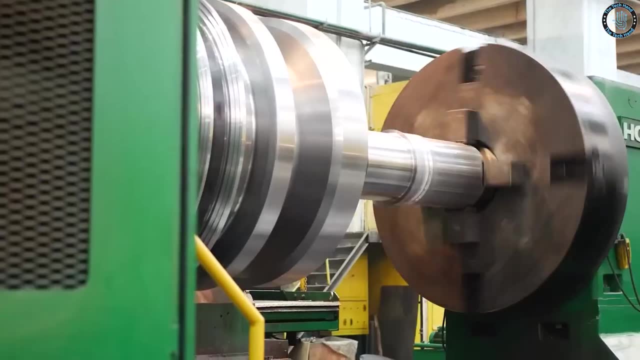 when scientists at the University of Cambridge in the UK discovered that when deuterium is fused with another deuterium nucleus, it can release a large amount of energy, This was the first experimental evidence that nuclear fusion could be a viable energy source. How Does Nuclear Fusion Occur? 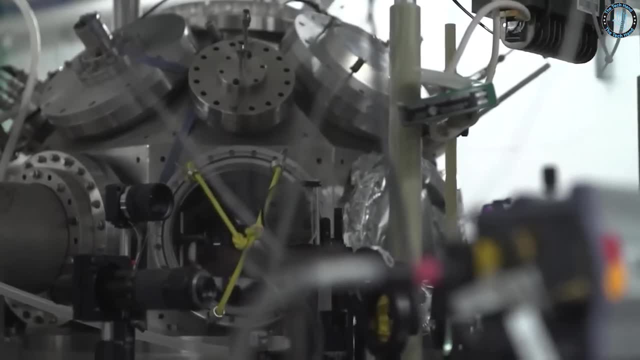 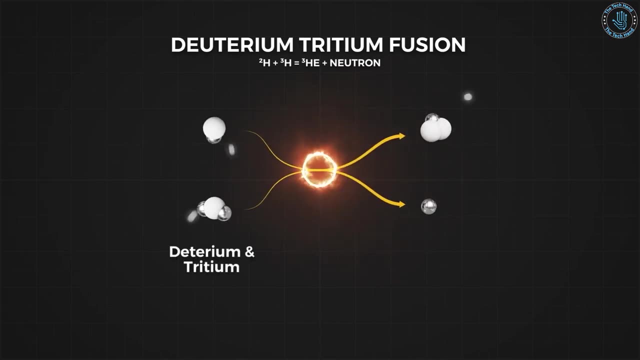 In order to achieve nuclear fusion, the positively charged nuclei of the atoms need to be brought close enough to each other that the strong nuclear force can hold them together. However, the positively charged nuclei will also repel each other due to the electrostatic force. 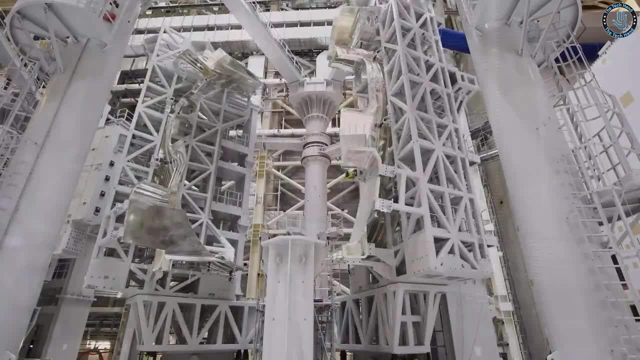 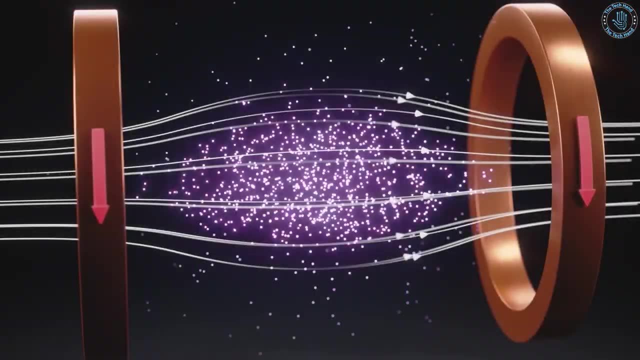 To overcome this repulsion, the atoms need to be heated to extremely high temperatures, on the order of millions of degrees, So that their nuclei are moving fast enough that they can overcome the electrostatic repulsion and come together. Additionally, the atoms need to be placed under extremely high pressures so that the 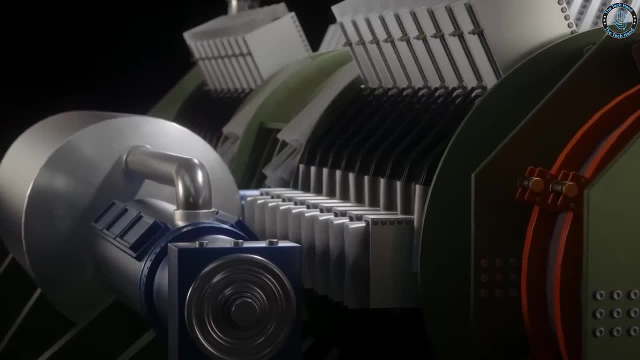 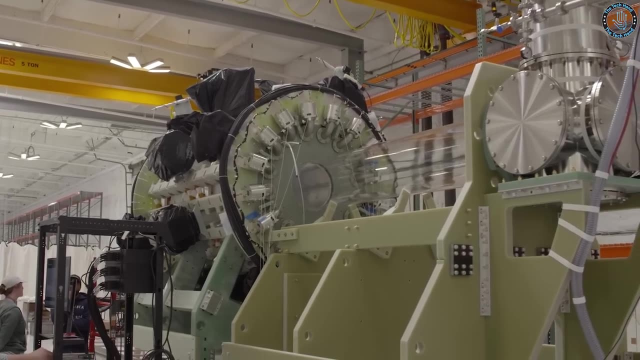 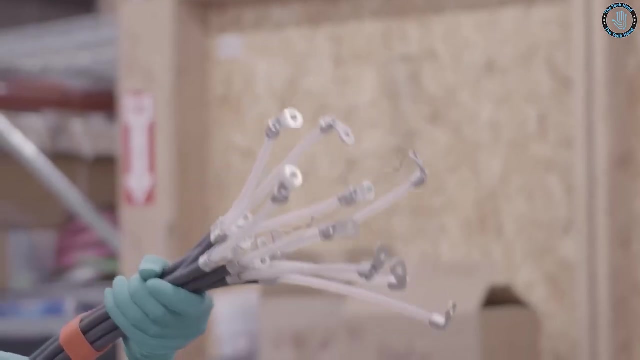 nuclei are squeezed together even more. The same principles can be used in a controlled environment like a nuclear fusion power plant. Researchers have been trying to create experimental reactors that can achieve the conditions necessary for nuclear fusion. These experiments have been ongoing for several decades, and, while a significant process has 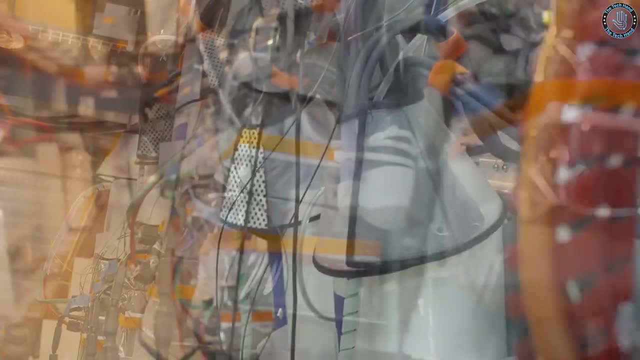 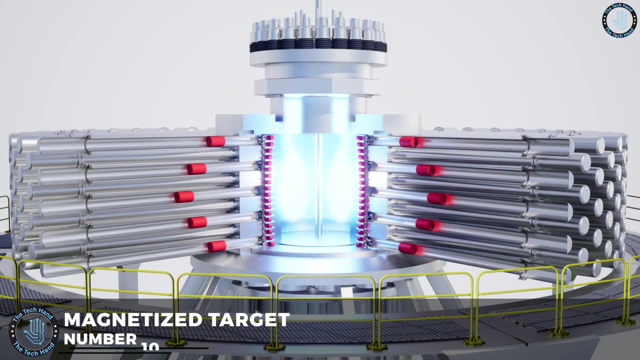 been made. there are still many technical challenges that need to be overcome before nuclear fusion. Here are some of the new ways to achieve nuclear fusion: Number 10. Magnetized target fusion. Magnetized target fusion is a fusion energy concept that combines aspects of magnetic 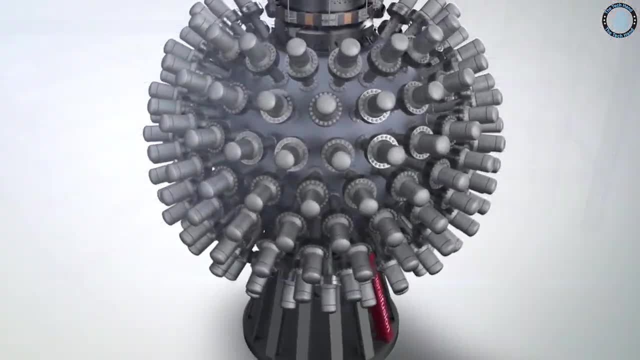 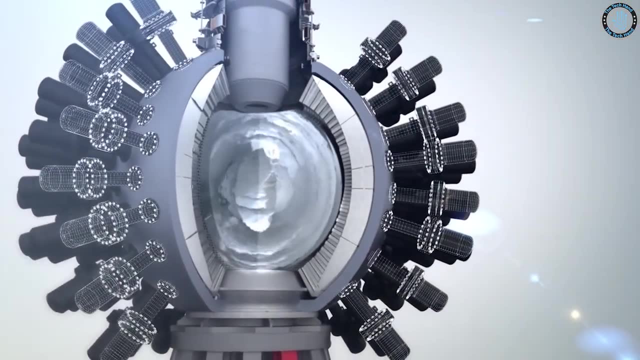 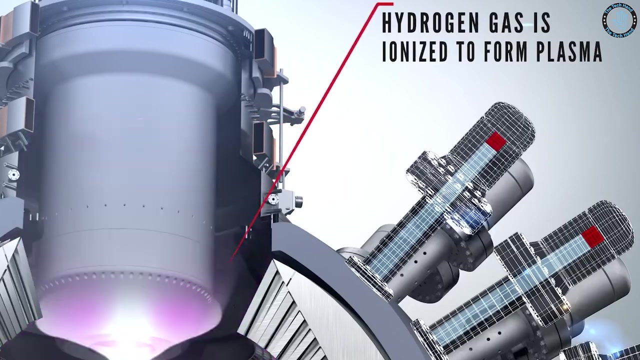 confinement and inertial confinement fusion. It involves using a combination of magnetic fields and high-energy lasers or particle beams to compress and heat the fuel With the goal of achieving a self-sustaining fusion reaction. In MTF, The fuel is contained in a small magnetized target that is suspended within a larger magnetic 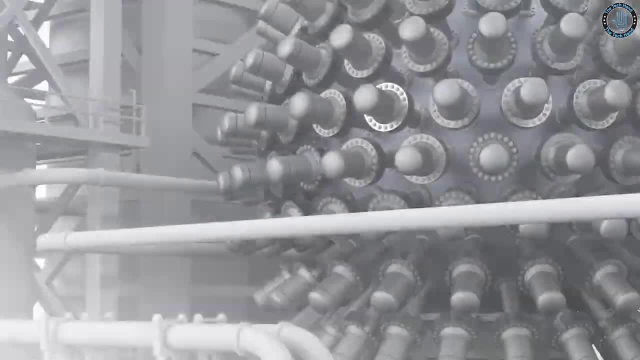 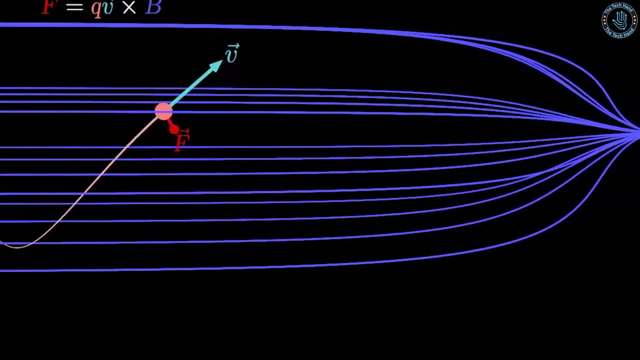 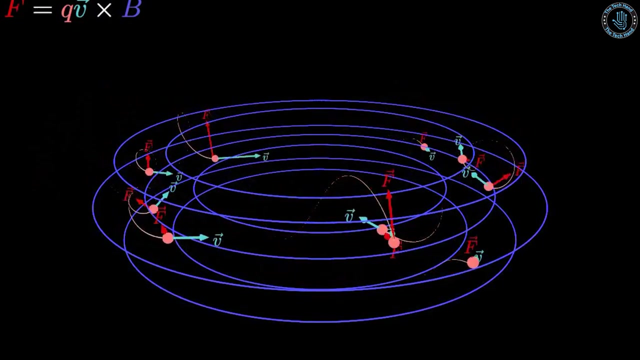 field. The target is then subjected to high-energy beams of particles or lasers, which heat and compress it, causing the fuel to ignite into a plasma. One of the main benefits of MTF is that it has the potential to achieve fusion at lower temperatures and pressures than are required by other approaches such as tokamaks and. 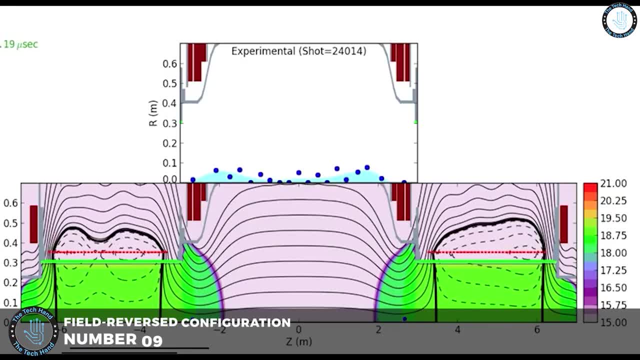 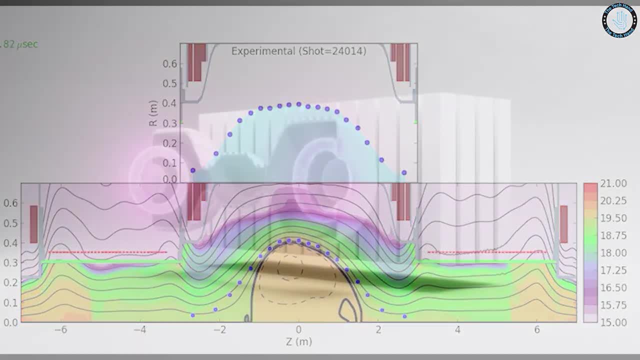 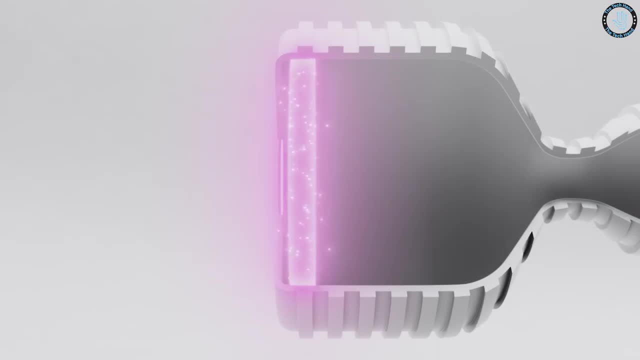 inertial confinement fusion. Number 9: Field Reverse Configuration: Fusion- Field reverse configuration. fusion is a fusion energy concept that involves creating a plasma with a special magnetic field configuration that allows it to sustain a fusion reaction for a longer period of time. In FRC fusion, a plasma is created by heating and ionizing a gas using electrical current. 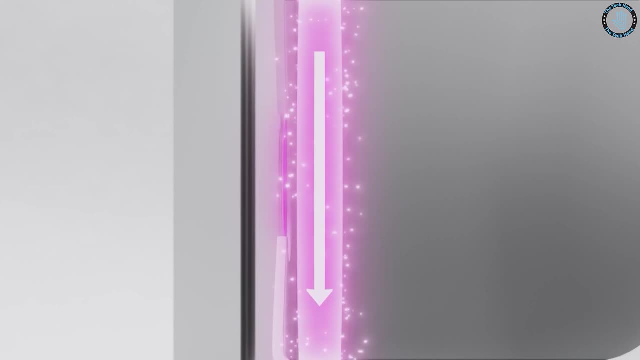 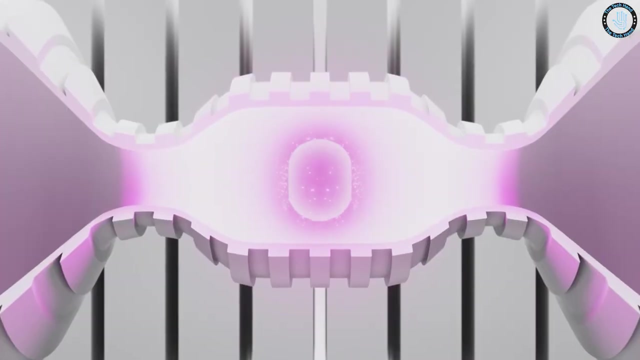 or a high-energy beam of particles or lasers. The plasma is then confined within a magnetic field that has a particle configuration known as a field reverse configuration, Or FRC. This configuration allows the plasma to sustain itself for a longer period of time, potentially. 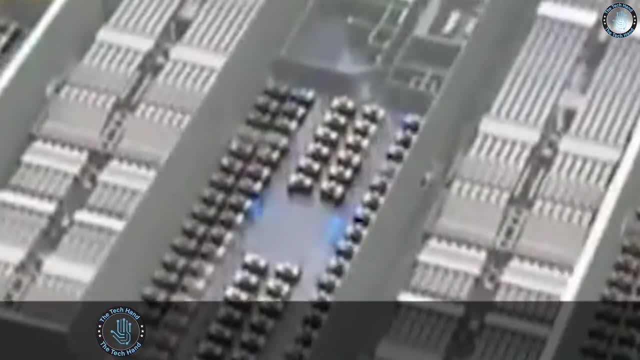 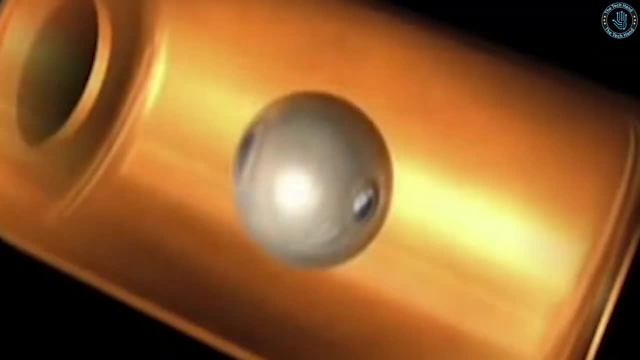 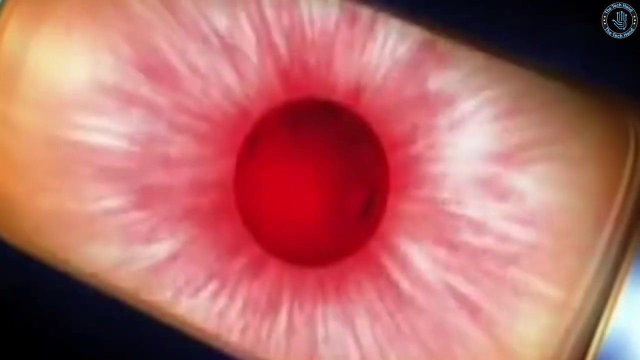 allowing for a more efficient and stable fusion reaction. Number 8: Laser Induced Plasma Acceleration Fusion. Laser Induced Plasma Acceleration fusion is a fusion energy concept that involves using high-energy lasers to accelerate a stream of plasma, causing it to collide and fuse. 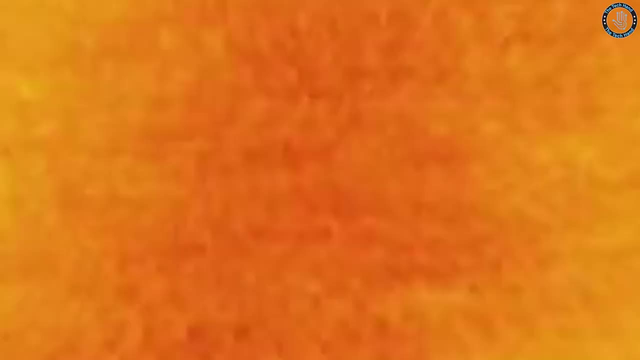 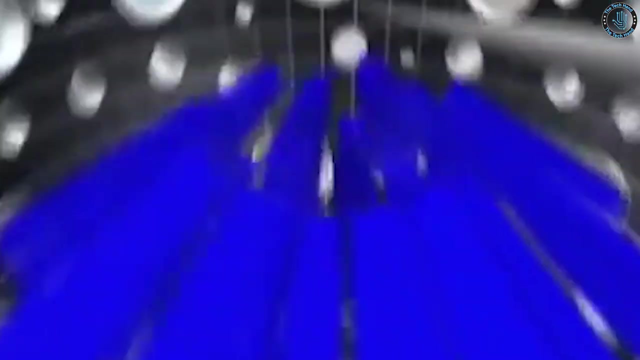 with another stream of plasma. In LIPA fusion, a gas is ionized using lasers To create a plasma. the plasma is then subjected to additional high-energy lasers which accelerate it to extremely high speeds. The accelerated plasma is then directed to collide with another stream of plasma, causing 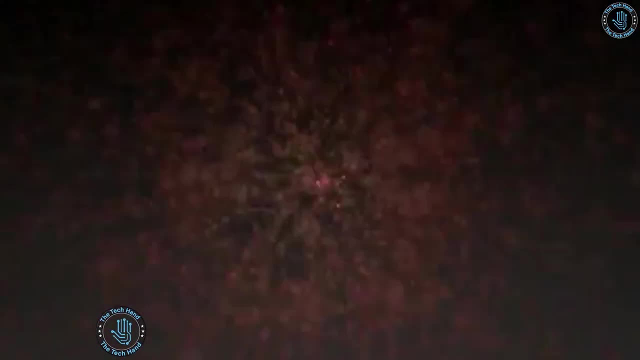 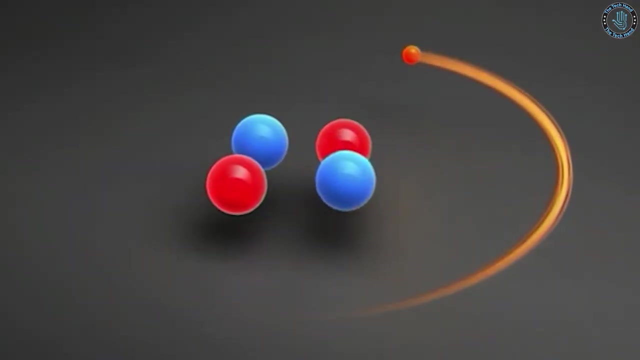 the two to fuse together and release energy. Number 7: Muon Catalyzed Fusion. Muon catalyzed fusion is a fusion energy concept that involves using subatomic particles called muons to catalyze the fusion of hydrogen isotopes, potentially at lower temperatures and pressures. 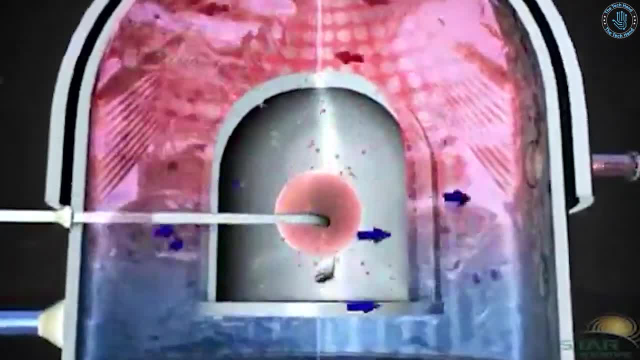 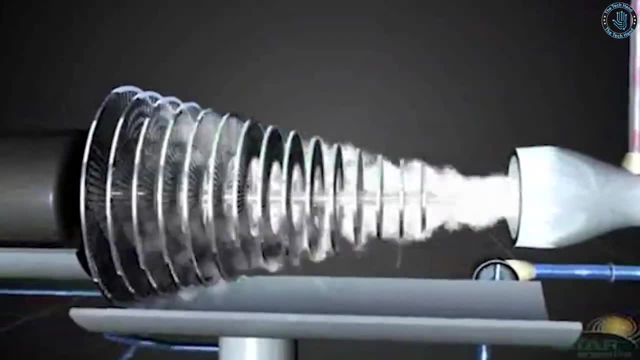 than are required for other approaches. In muon catalyzed fusion, a gas is cooled to extremely low temperatures, at which point it can be converted into a solid or liquid state. Muons, which are subatomic particles with a positive charge, are then introduced into. 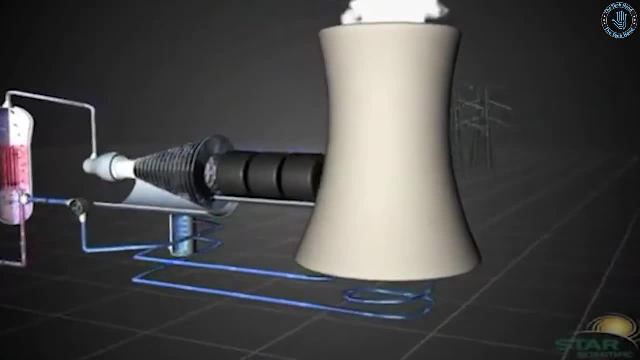 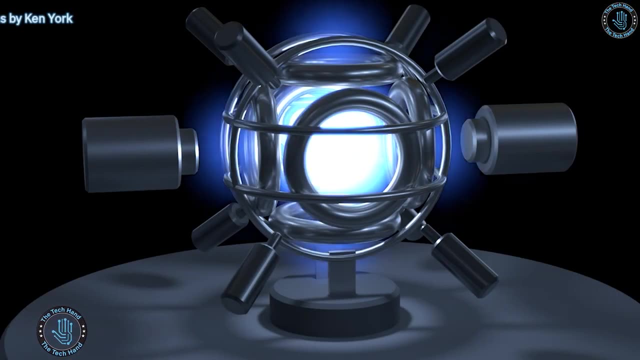 the fuel. The muons can interact with the hydrogen nuclei, causing them to fuse together and release energy. Number 6: Polywell Fusion. Polywell fusion is a fusion energy concept that uses a combination of electric and magnetic fields to confine and heat a plasma. 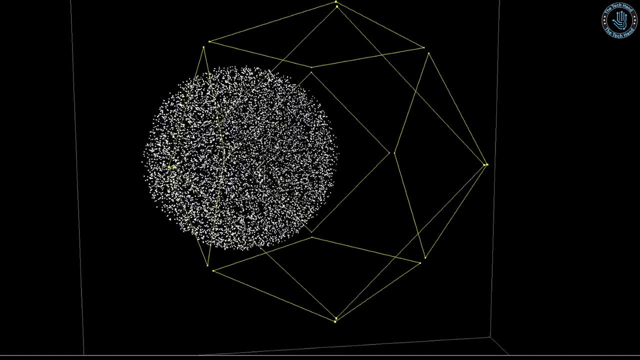 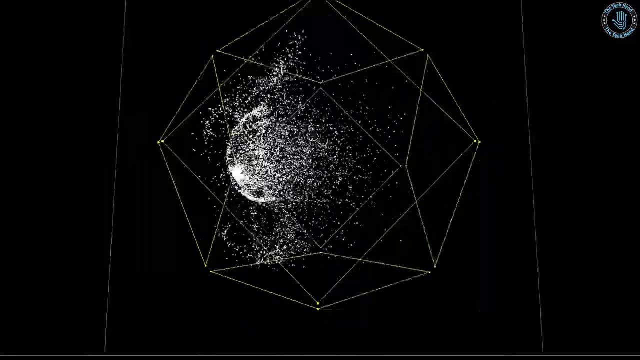 With the goal of achieving a self-sustaining fusion reaction. In polywell fusion, a gas is ionized using an electric current to create a plasma. The plasma is then confined within a complex arrangement of electric and magnetic fields known as a polywell. 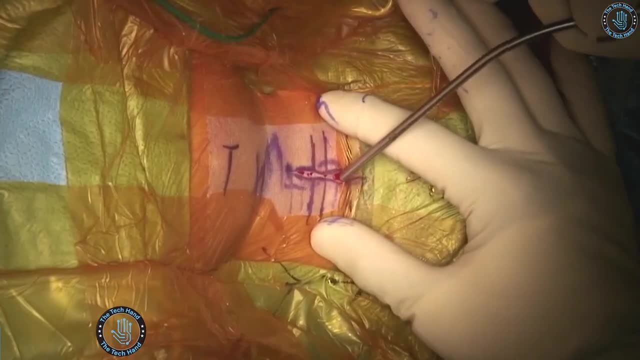 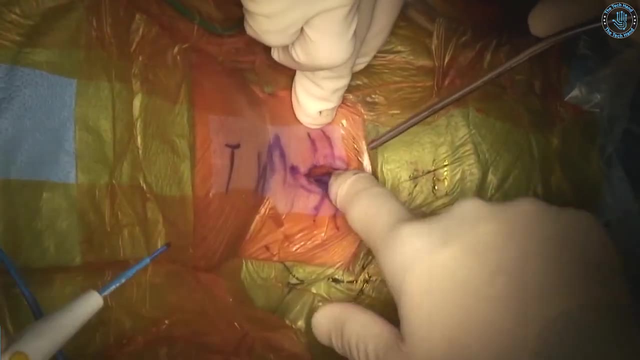 The fields are used to heat and compress the plasma. Number 5: C2U Fusion. C2U fusion is a fusion energy concept that involves using a combination of lasers and an electric field to compress and heat the fuel, causing it to ignite into a plasma. 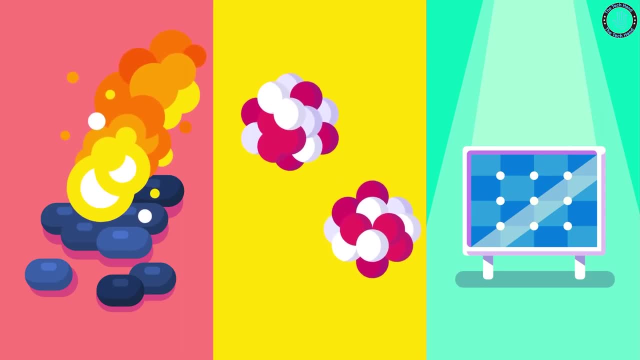 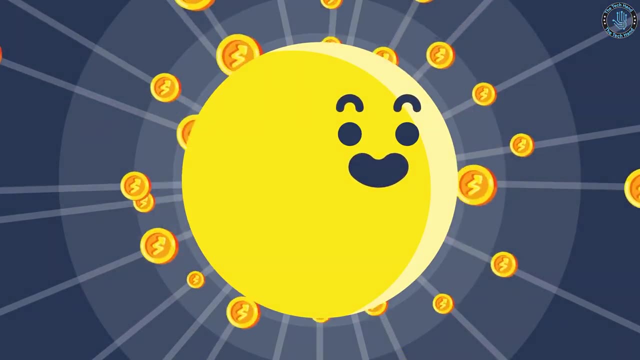 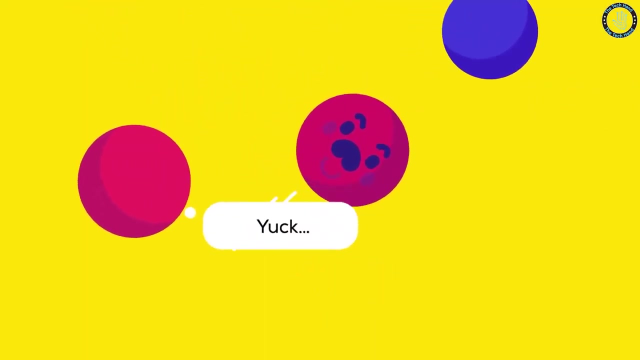 In C2U fusion, a gas is ionized using an electric current to create a plasma. The plasma is then subjected to high-energy lasers, which heat and compress it, causing the hydrogen nuclei to fuse together and release energy. One of the main benefits of C2U fusion is that it has the potential to achieve fusion. 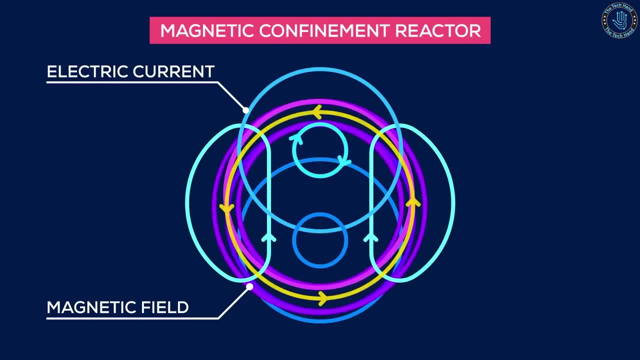 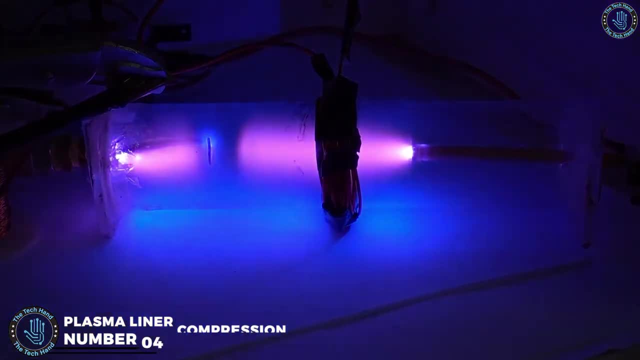 at relatively low temperatures and pressures, potentially making it a more efficient and cost-effective approach. Number 4: Plasma Liner Compression Fusion. Plasma liner compression fusion is a fusion energy concept that uses a combination of electric and magnetic fields to create a plasma. This fusion energy concept that involves using a plasma liner to compress and heat the fuel. 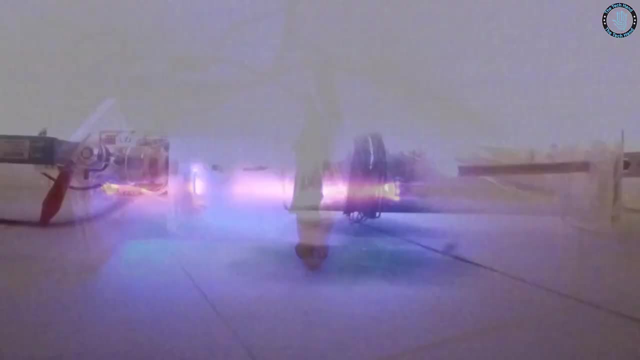 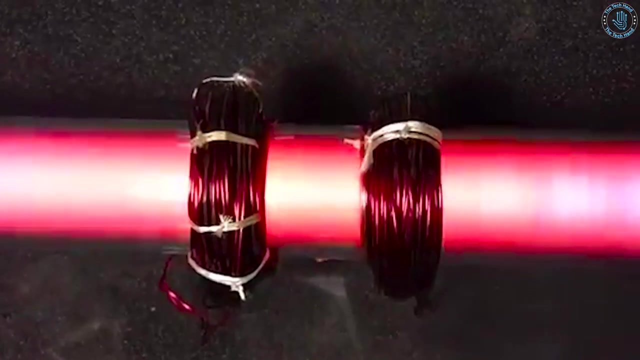 causing it to ignite into a plasma. In plasma liner compression fusion, a gas is ionized using an electric current or a high-energy beam of particles or lasers to create a plasma. The plasma is then confined within a plasma liner, which is a shell of plasma that is 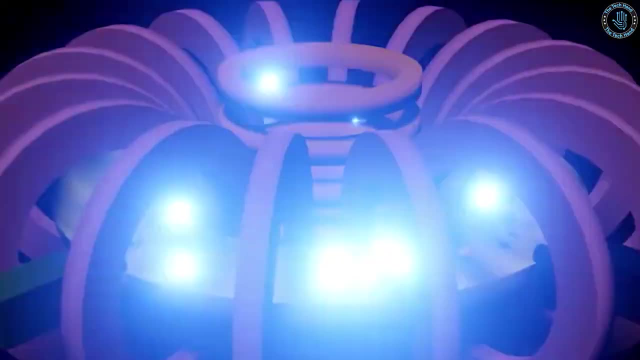 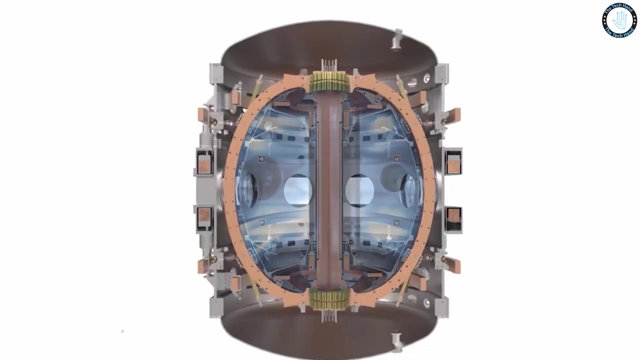 used to compress and heat the fuel, causing it to ignite into a plasma. Number 3: M-Biosferical Tokamak. M-Biosferical Tokamak is a fusion energy apparatus that is used to create energy into. is a variant of a tokamak fusion device that uses a specially shaped magnetic field to confine the 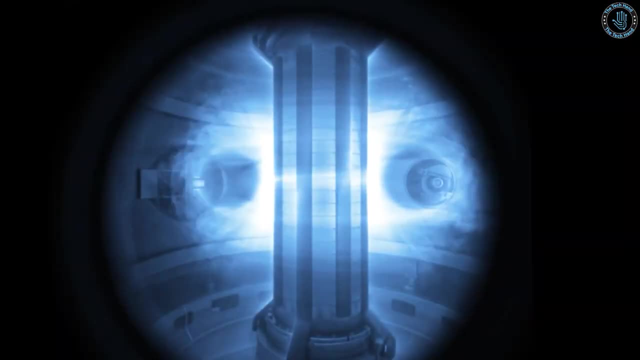 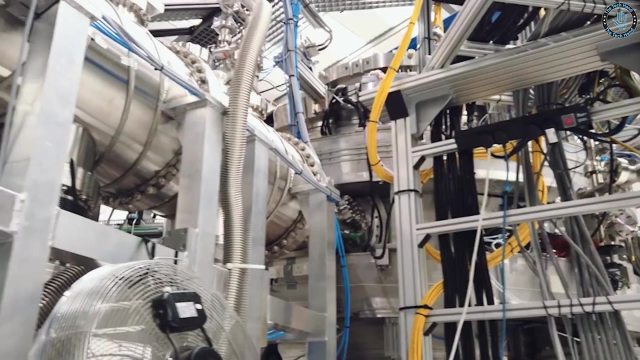 plasma and stabilize the fusion reaction. In a tokamak, the fuel is contained in a plasma within a toroidal magnetic field. The MST design modifies the shape of the magnetic field in order to improve the stability and performance of the plasma. Specifically, the MST design uses an 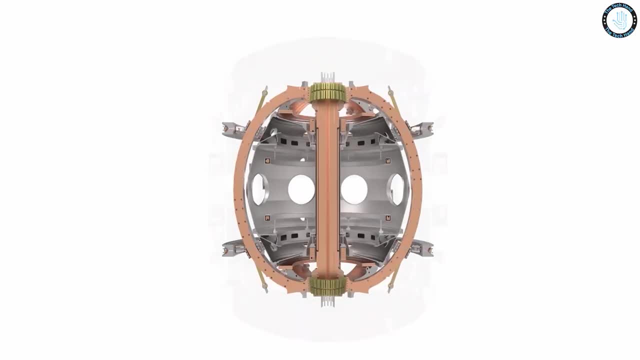 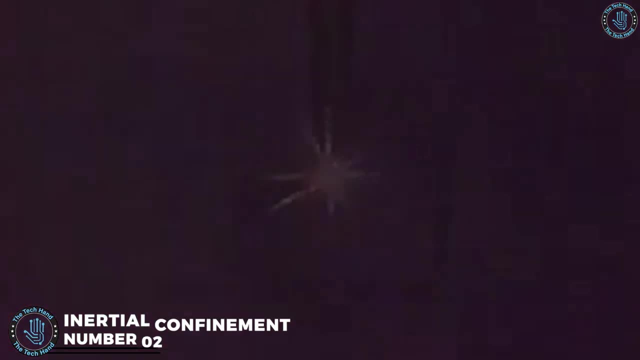 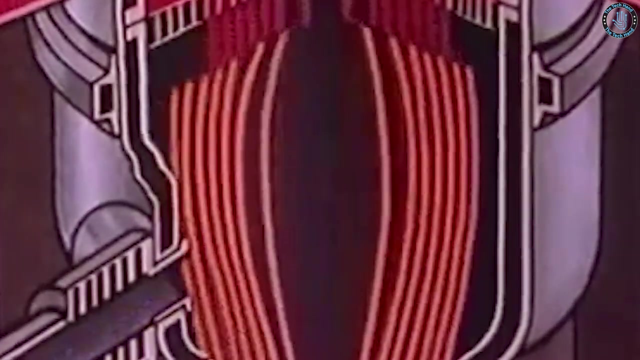 M-shaped magnetic field, which is created using a system of magnets arranged in a particular configuration. Number 2. Inertial Confinement Fusion. Inertial confinement fusion- ICF- is a fusion energy approach that involves using high-energy lasers and particle beams to compress and heat a small pallet of fuel, causing it to ignite into.